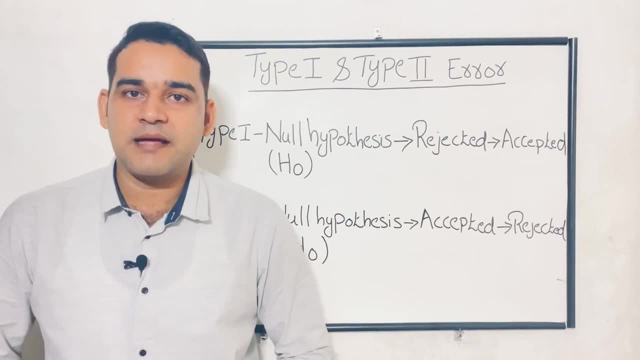 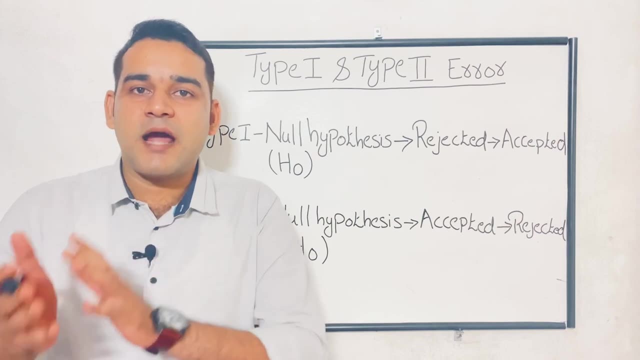 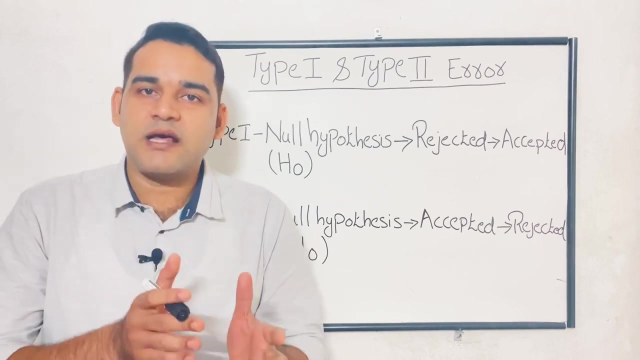 Hi everybody, I am Naufal. Welcome to my channel. Today we are going to discuss regarding type 1 and type 2 error. Most of the students are confused with these two terms, that is, type 1 and type 2 error. By watching this video, you will get an idea regarding what is type 1 error, as well as what is type 2 error. Before moving to the topic, you should know regarding what is null hypothesis. Then only you will get a better idea regarding type 1 and type 2 error. 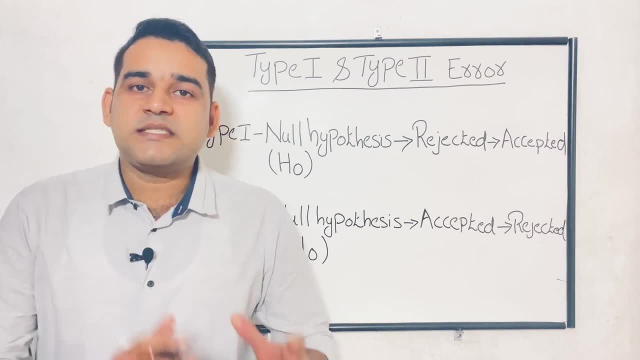 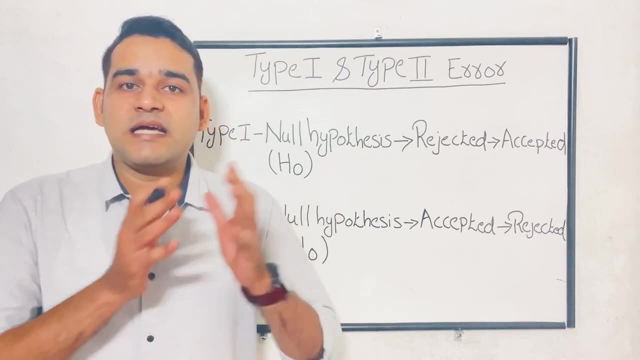 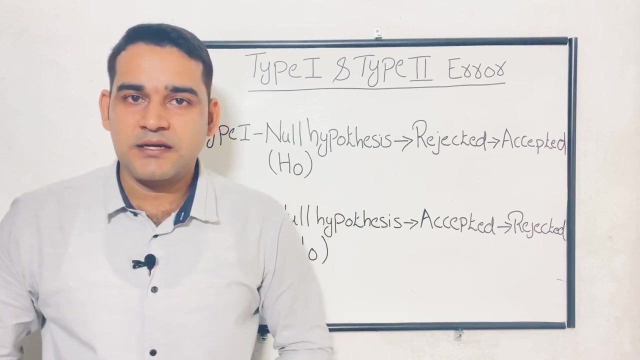 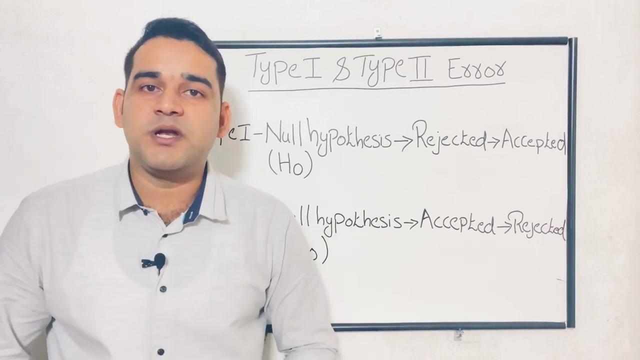 Let us see regarding null hypothesis. What is null hypothesis? Null hypothesis is a type of hypothesis which states that there is no relationship between independent and dependent variable. Null hypothesis is a type of hypothesis which states that there is no relationship. There is no relationship between independent as well as the dependent variable. 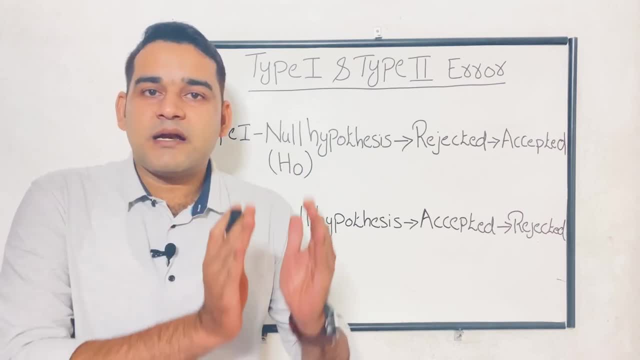 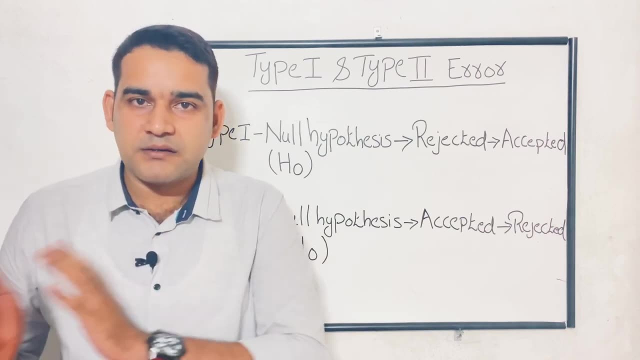 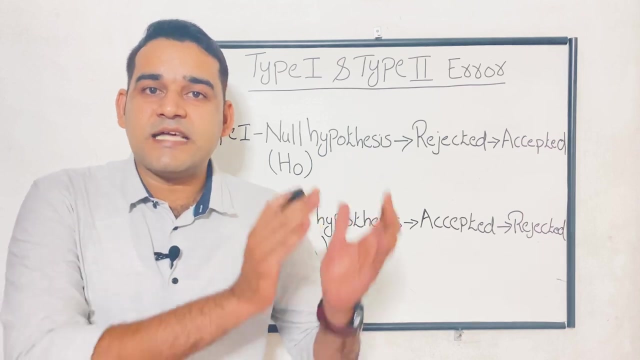 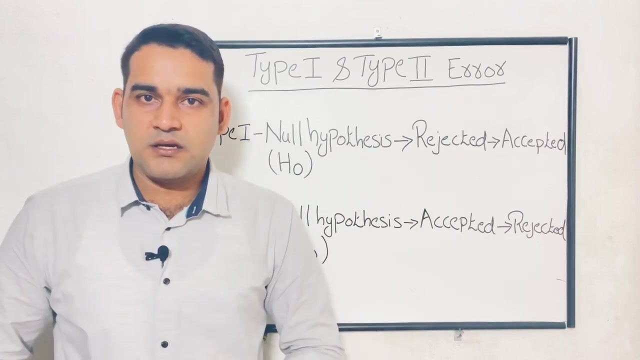 So you will get confused. I will give you a better example. There is no relationship between eating ice cream and back pain. This is a null hypothesis. There is no relationship between eating ice cream and back pain. It is a statement. It is a null hypothesis. If you want to know regarding hypothesis and the null hypothesis, I have already done a video on null hypothesis. 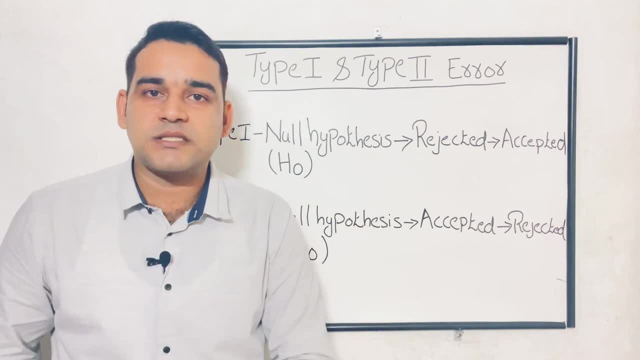 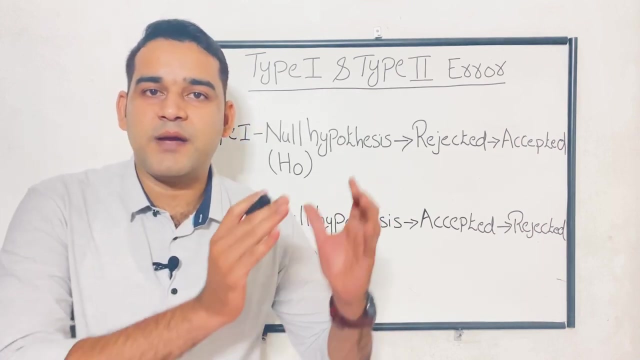 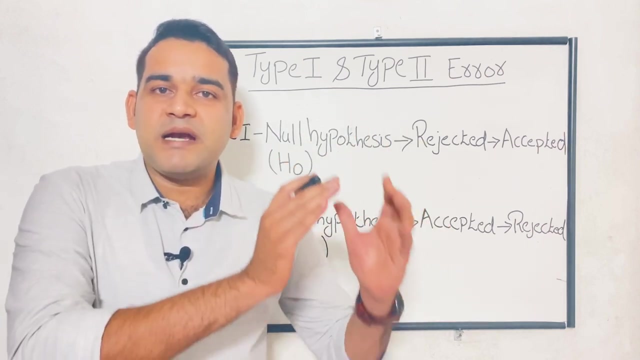 I will give the link in the description box. Just go through that So you will get an idea regarding what is hypothesis and what is null hypothesis. Now I will give a brief idea regarding null hypothesis. Null hypothesis is a type of hypothesis which states that there is no relationship between independent and dependent variable. 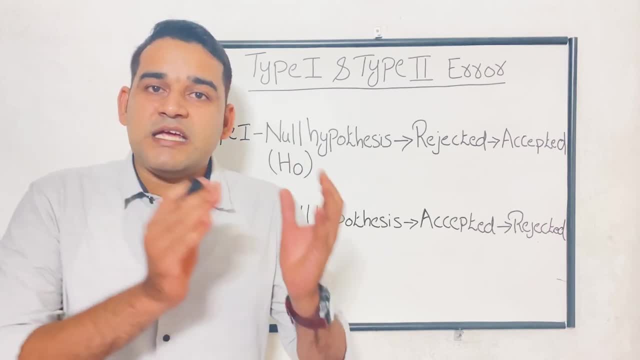 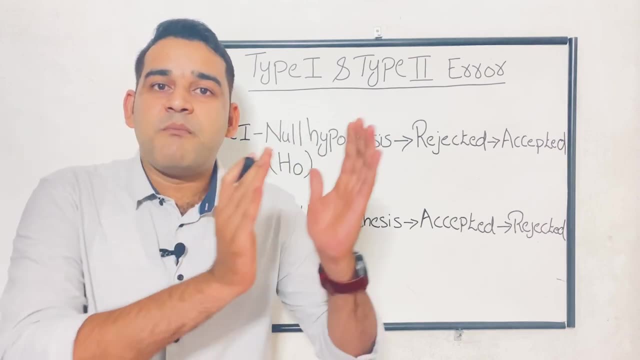 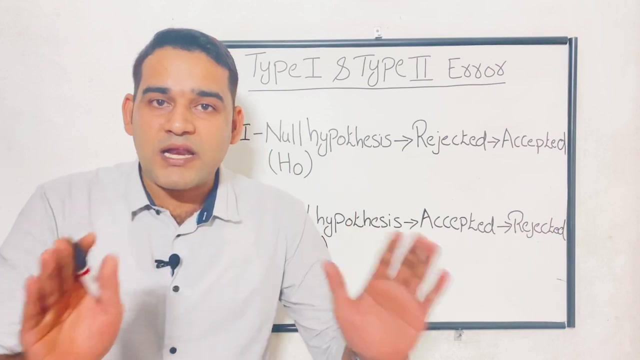 If you want to know, regarding hypothesis and the null hypothesis, Bong spoke about this. There is no relationship between independent and dependent variables. ice cream and back pain. there is no relationship between eating ice cream and back pain is a example of null hypothesis. it will always state that there is no relationship between independent. 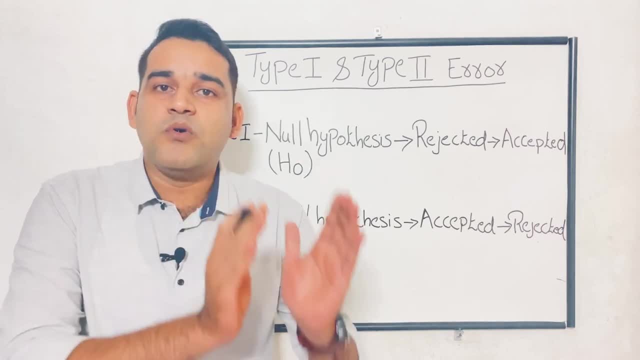 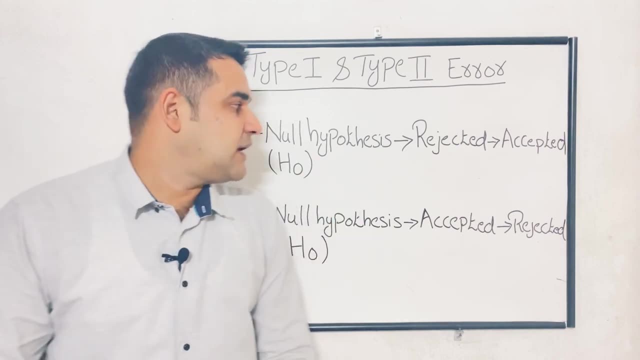 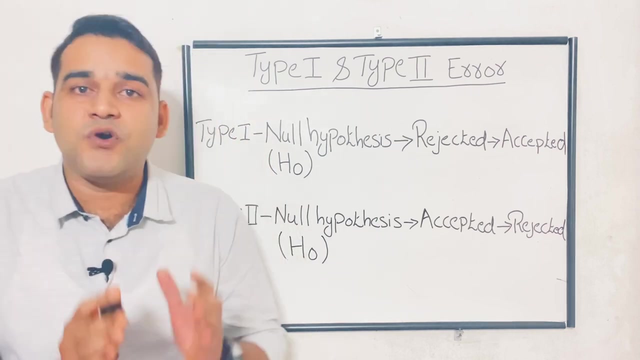 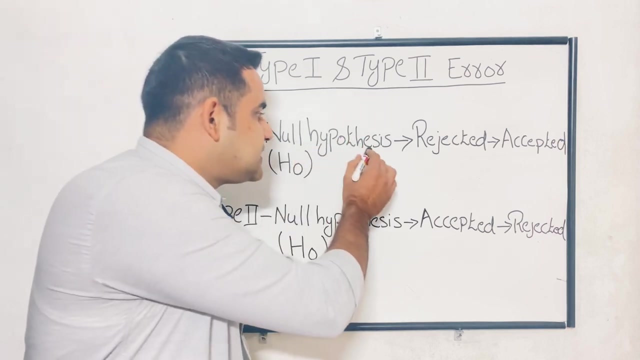 and dependent variable. now we can move to our topic, that is, type 1 error and type 2 error. okay, first one is type 1 error. so what is type 1 error actually? if you are a researcher, okay, if you are a researcher and a null hypothesis is there? okay, a null hypothesis is there actually? you have to. 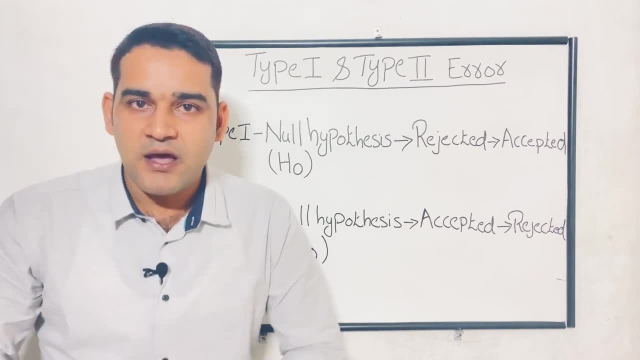 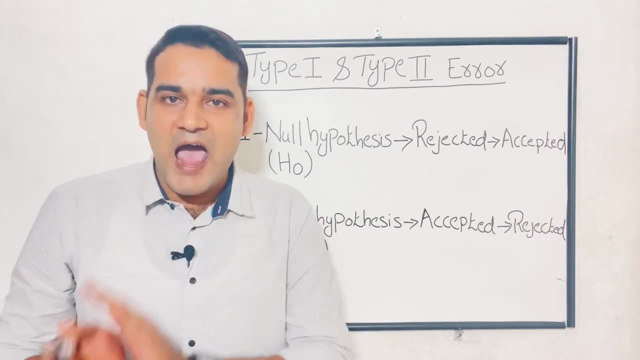 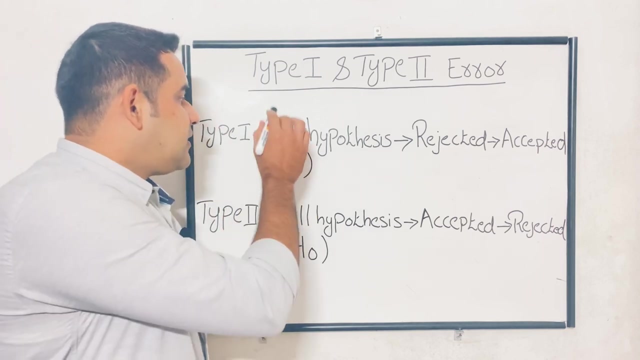 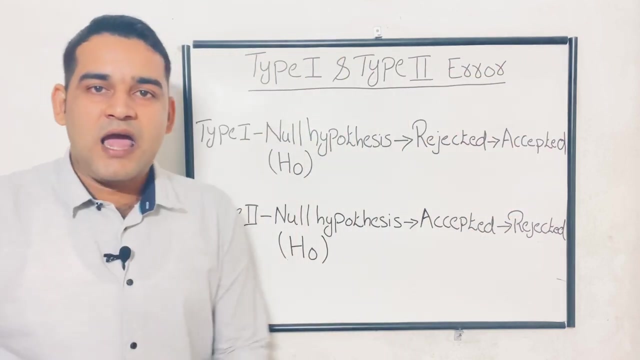 accept that null hypothesis. with our example eating, there is no relationship between eating ice cream and back pain. we know that there is no relationship between eating a ice cream and your back pain. there is no relationship at all. so here type 1 error will occur when, if the null hypothesis is rejected, actually you have to accept okay. 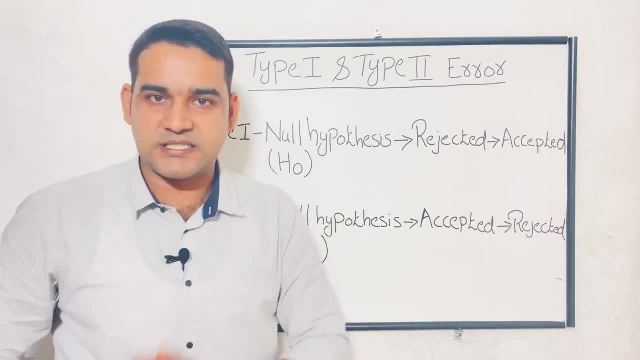 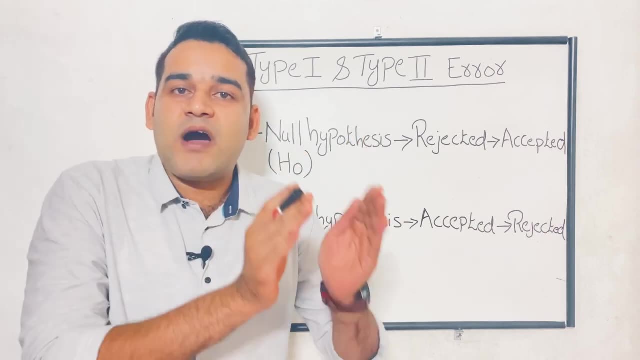 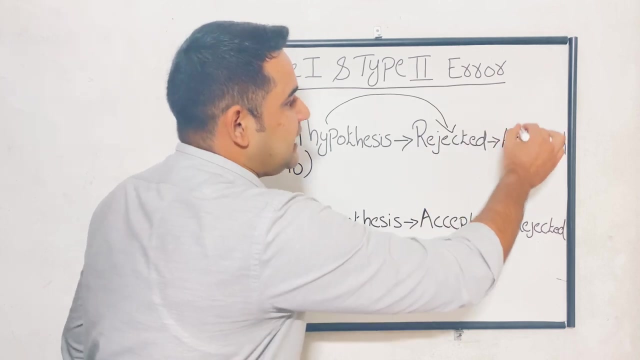 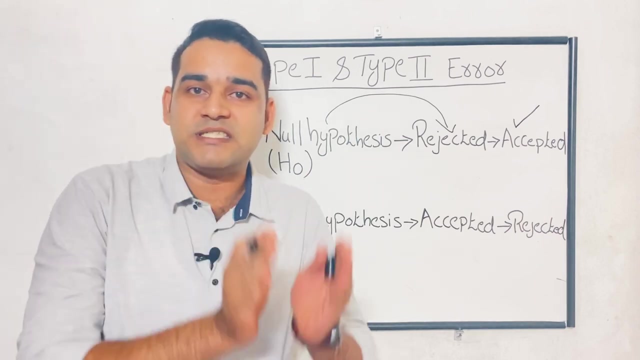 actually, you have to accept the null hypothesis. by mistake, what you have done, you have rejected. that time what will occur? type 1 error will occur. okay, a null hypothesis is rejected. actually, you should have been accepted. you have to accept actually, but by mistake you rejected the. 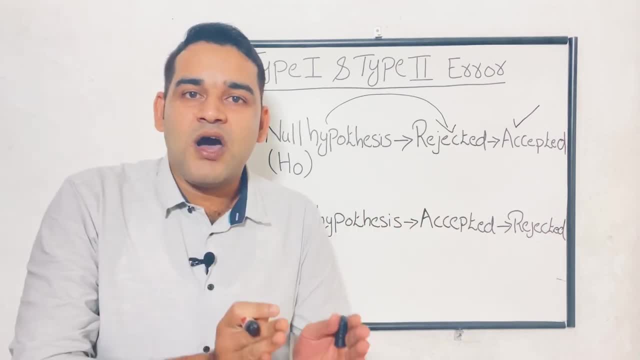 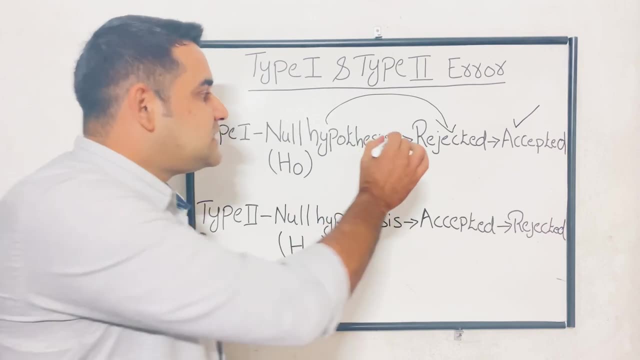 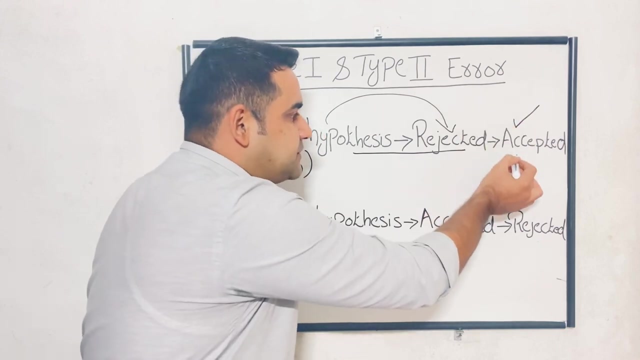 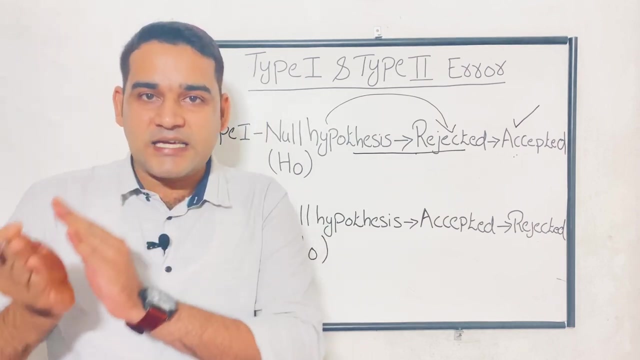 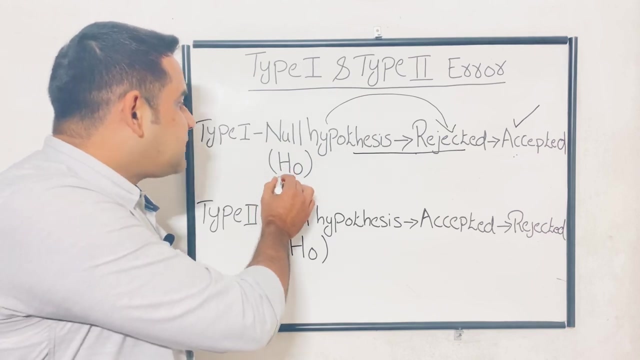 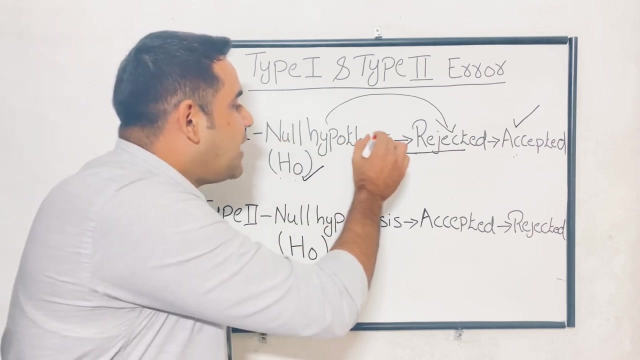 null hypothesis. our example is: there is no relationship between eating ice cream and back pain. by mistake, you rejected this null hypothesis. actually, you have to accept instead of accepting. you rejected the null hypothesis. okay, instead of accepting, you rejected the null hypothesis. this is the symbol of the null hypothesis. that is h knot. okay, h knot is the symbol of the null hypothesis. so type 1 error will occur when a null hypothesis is rejected. actually it should have been accepted. actually you have to accept the null hypothesis, but by mistake you rejected, type 1 error will occur. So what is type 2 error? Type 2 error is just opposite to type 1 error. Here, instead of rejecting a null hypothesis, you accept it. 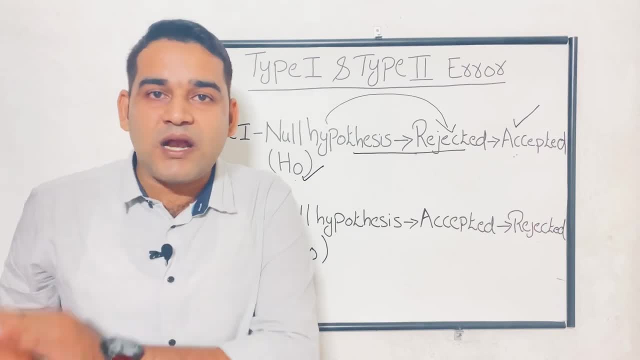 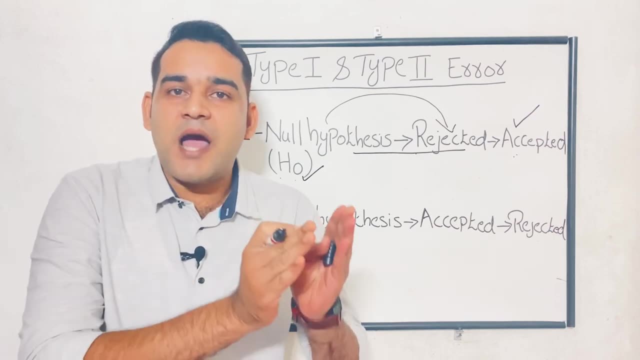 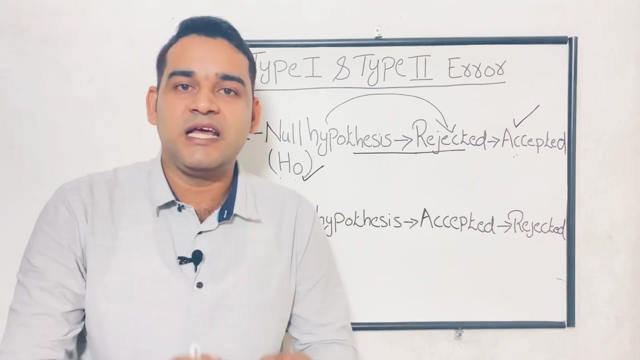 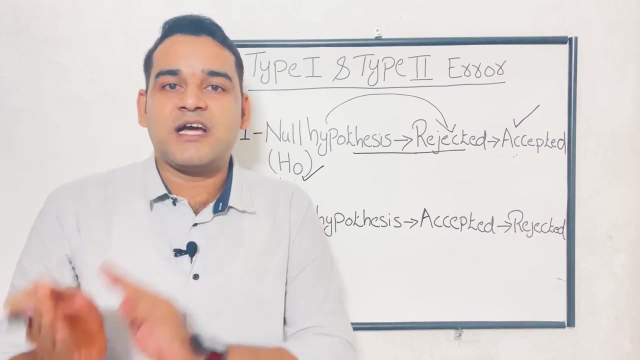 For example, there is no relationship between eating ice cream and throat pain. This is a null hypothesis. There is no relationship between eating ice cream and throat pain. Actually, there is relationship between eating ice cream and throat pain because for some children, they will get throat pain after taking the ice cream. 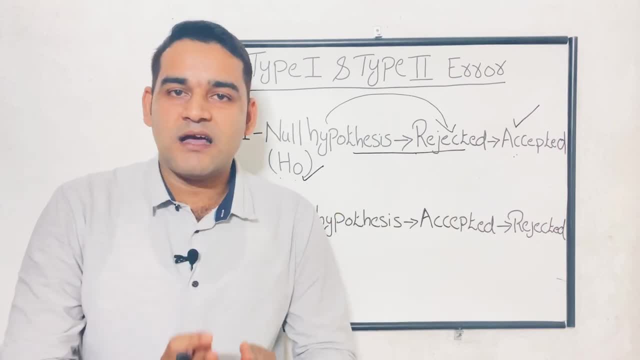 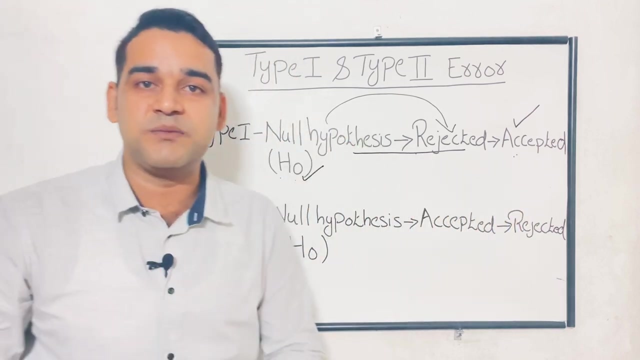 Our example in the null hypothesis is: there is: There is no relationship between eating ice cream and throat pain. for the type 2 error. Our null hypothesis is: there is no relationship between eating ice cream and throat pain. So if you are a researcher, actually you have to reject this. There is no relationship between eating ice cream and your throat pain. Actually, you have to reject. 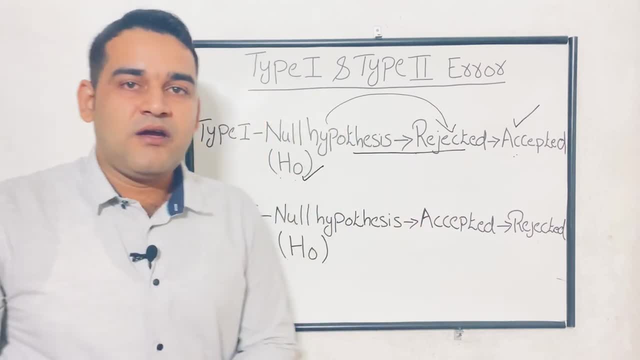 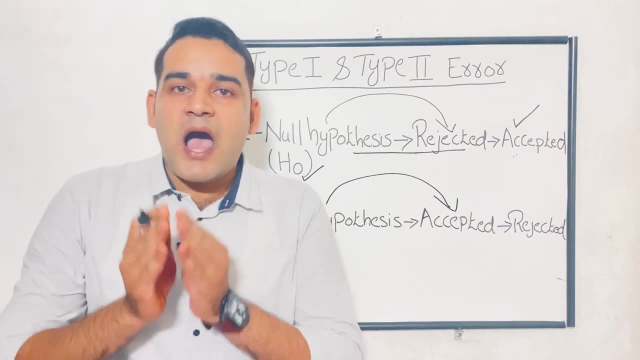 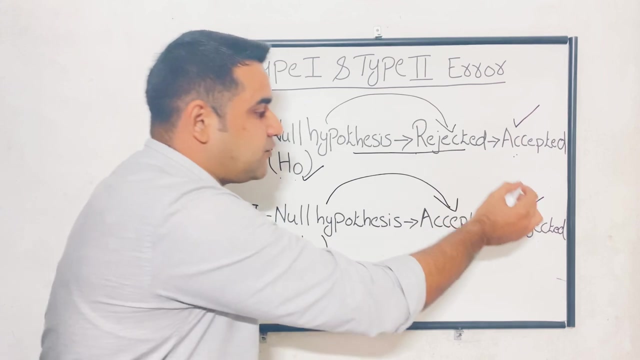 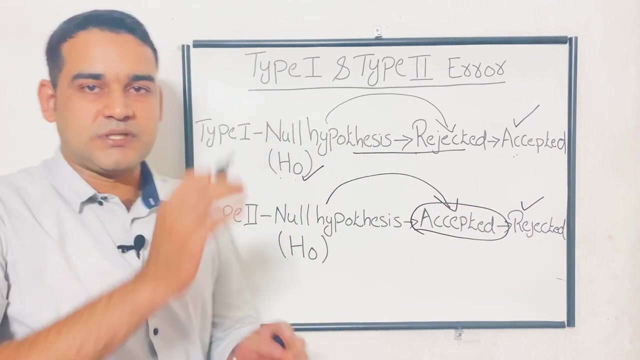 But what you have done? You accepted. Okay, When a null hypothesis is accepted, actually it should have been rejected. Okay, Just opposite to type 1.. Here, what you have to do, Actually you have to reject, But by mistake, you accepted the null hypothesis. 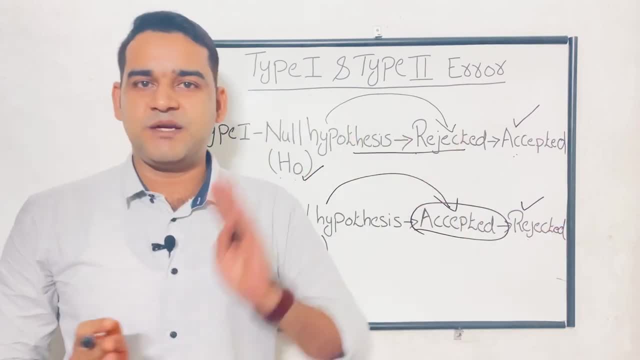 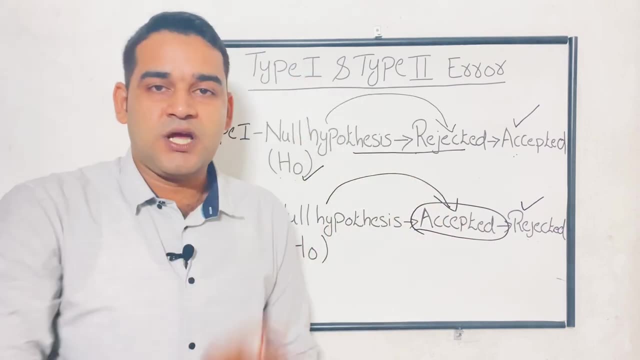 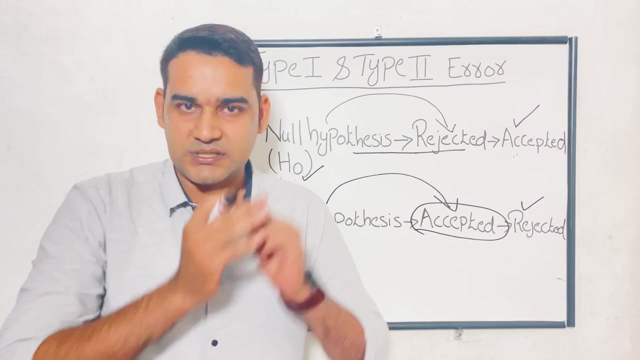 Okay, Actually, what you have to do, You have to reject that statement, You have to reject that null hypothesis. But, by mistake, What you have done, You accepted, You accepted a null hypothesis. Actually, you have to reject that null hypothesis. 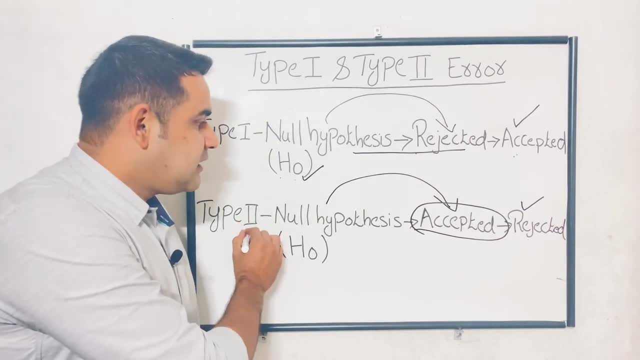 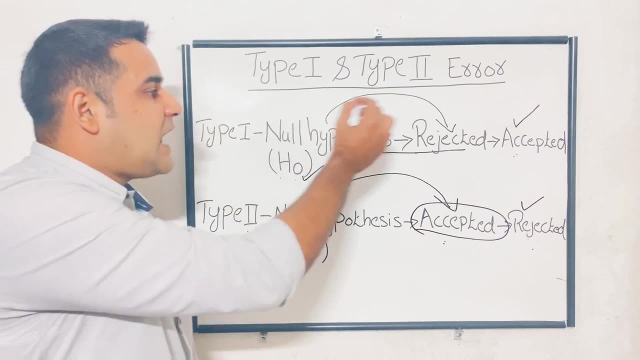 Okay, So type 2 error occurred Here. you have accepted It was a wrong decision. Actually, you have to reject In the type 1, the right decision is you have to accept the null hypothesis. By mistake you rejected. 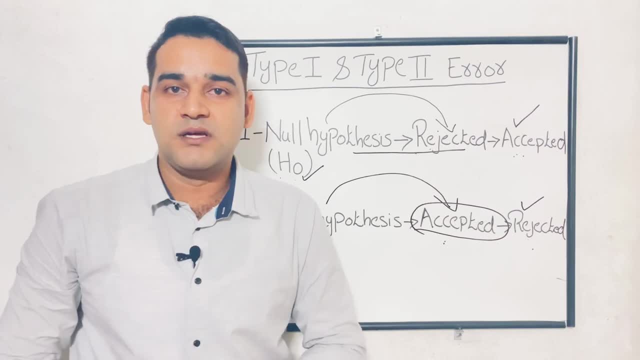 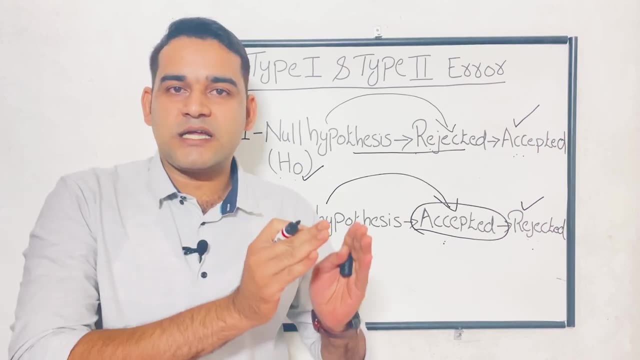 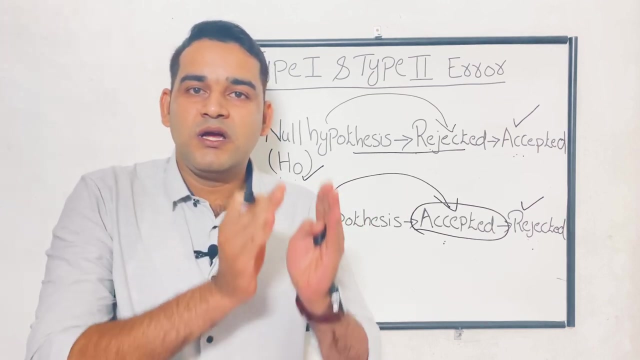 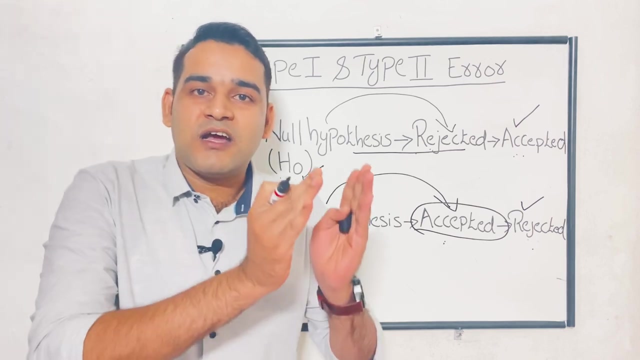 Got it Now I will give you a simple, Simple example So you will get a better idea regarding type 1 and type 2 error. Okay, After completing the course, you got a very good job offer. Okay, You got a very good job offer with high salary, less working time, good working condition. 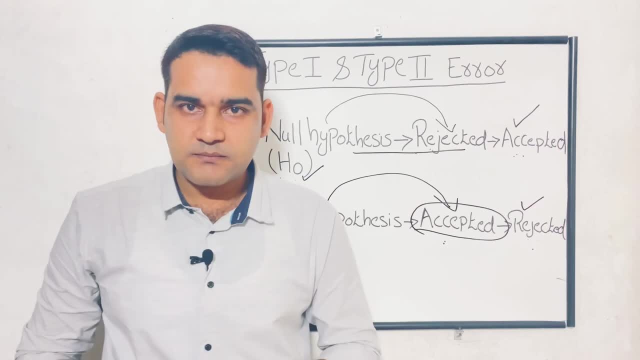 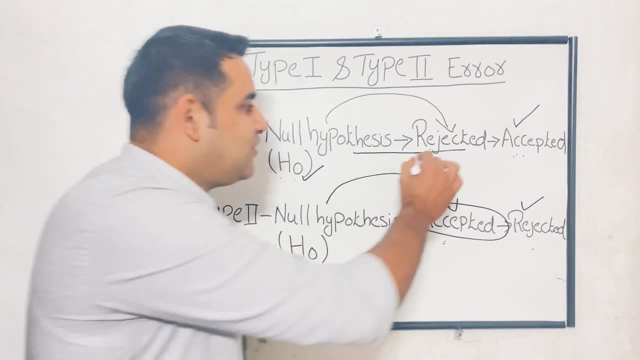 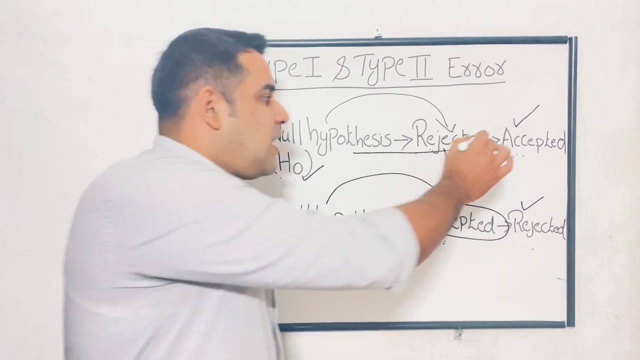 Okay, You got a very good job offer, But you thought that it is not a good job offer. But you thought that it is not a good job offer. So, by mistake, what you have done, You rejected your job offer. Actually, what you have to do, You have to accept. 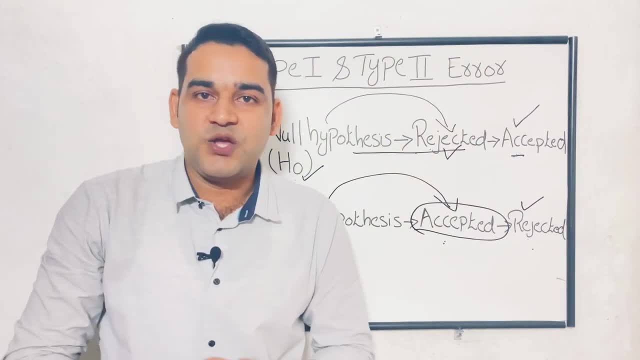 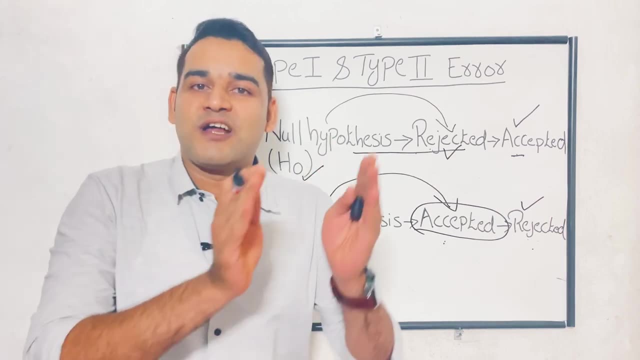 Okay, It was a good job offer. By mistake, you rejected Actually what you have to do: You have to accept. Instead of accepting that job offer, you rejected What happened. Type 1 error. Type 1 error.